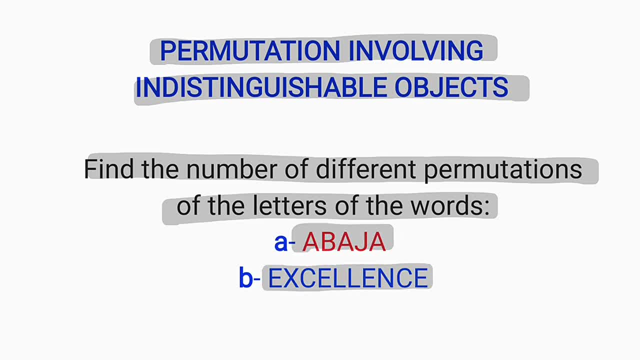 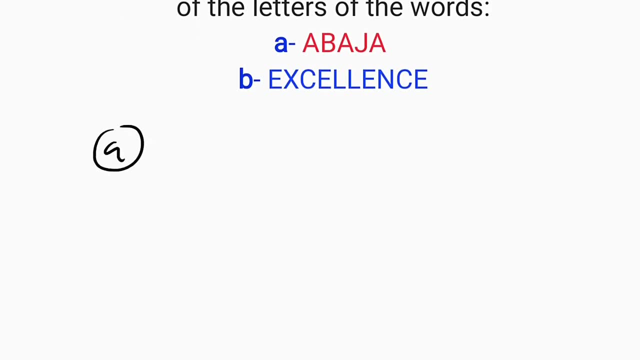 abadja and excellence. Okay, let's start with the first one, abadja. The first question. we want to find the different ways of arranging the letters of the word abadja. Abadja is a five letter word. I remember that we have n- factorial. 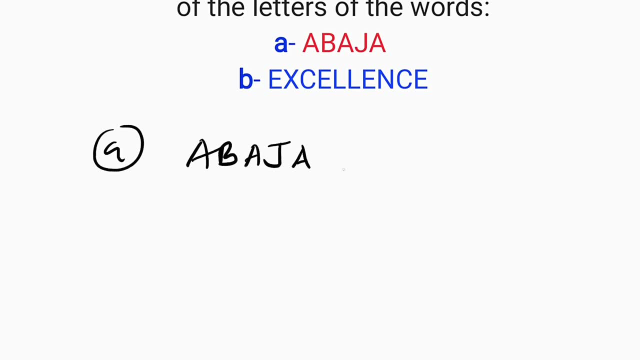 different ways of arranging n objects. Therefore, since we have n equal to five here, we have n factorial ways of arranging abadja. But there is a problem because we have three identical letters: We have one here, the other one here and 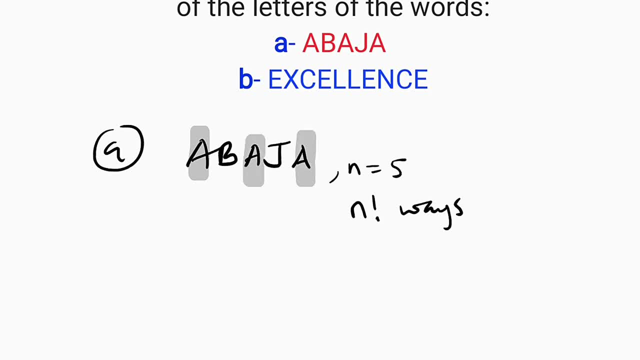 the other one. here You cannot differentiate by swapping the letters. Suppose I decide to take this one to this direction and I bring this one backward: A is E, no matter where you take it to. So you cannot differentiate it. Hence we are going to divide by the number of ways we can arrange E's in this. 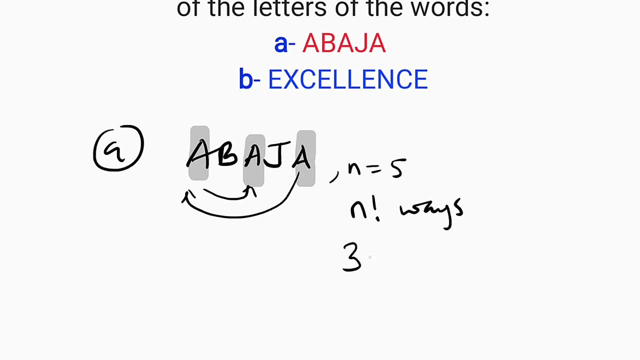 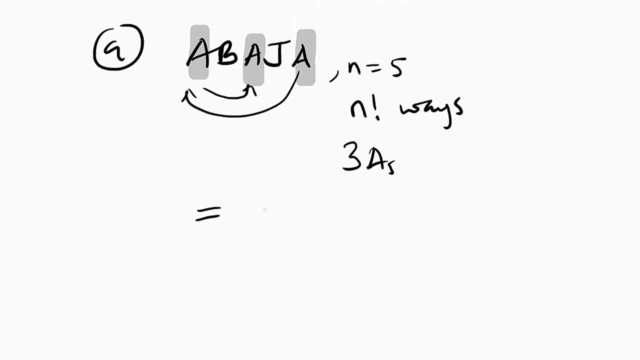 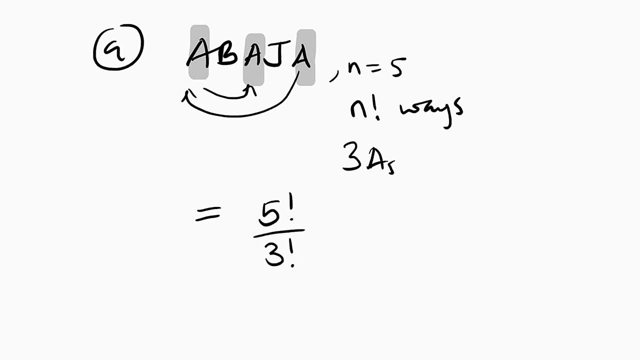 divided by three factorial. And three factorial stands for the number of ways we can arrange E's, since we cannot differentiate them. This is equal to 5 multiplied by 4, multiplied by 3, multiplied by 2, multiplied by 1, for 5 factorial divided by 3 factorial. 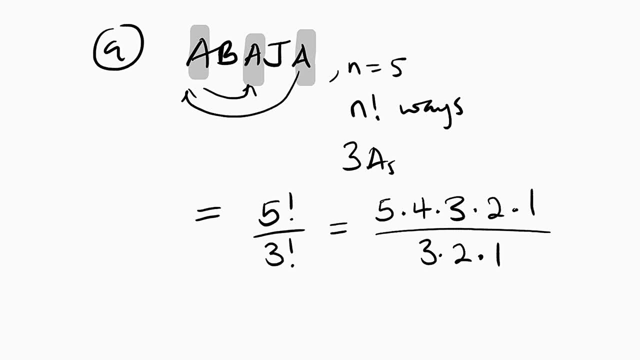 This is equal to 3 multiplied by 3, multiplied by 2, multiplied by 1 for 5.. So, from here, 3, 2, 1 will cancel 3, 2, 1.. All we have left is 5 multiplied by 4, which is equal to 20.. 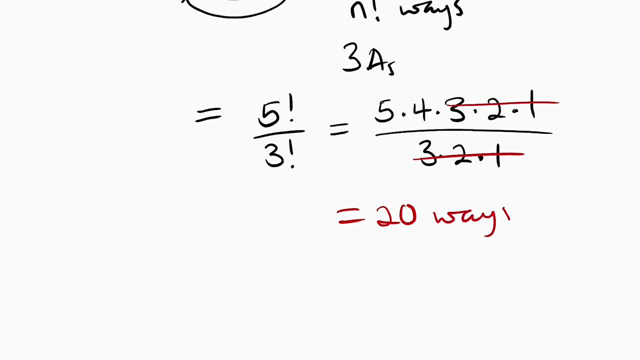 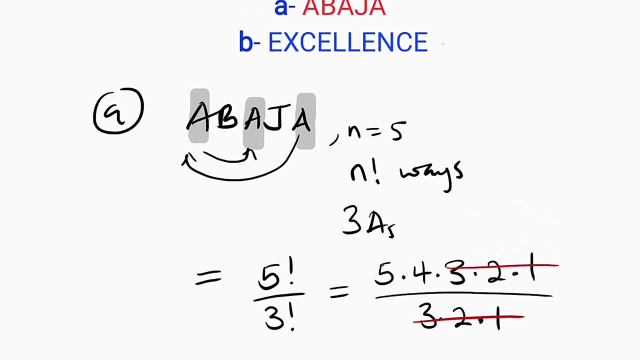 So we have 20 different ways of arranging the letters of the word abadja, considering E's that are identical. So now let us consider B, which is excellence. So now, let us consider B, which is excellence. So now let us consider B, which is excellence. 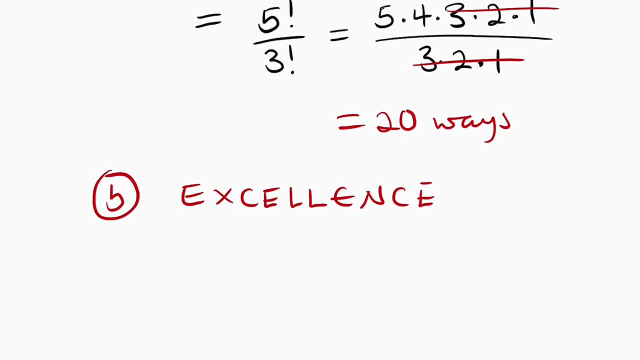 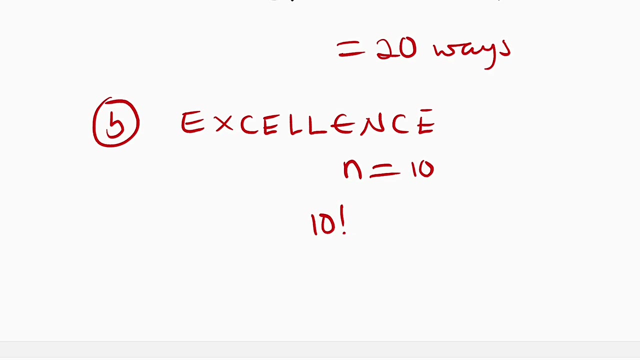 All right, as you can see, we have 10 letters. All right, as you can see, we have 10 letters and excellence, therefore n equal to 10, and we have 10 factorial different ways of arranging 10 objects. but we have a problem again because, you can see, we 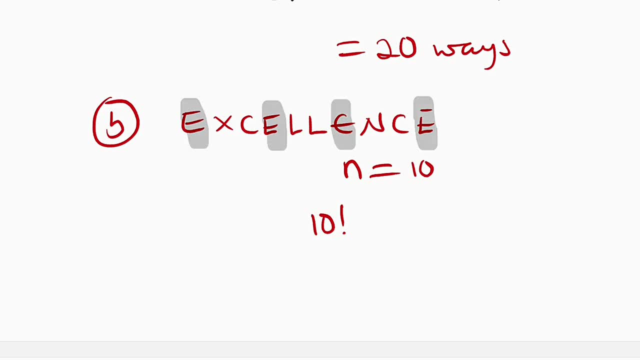 have e, e, e, e, and all of these e's are identical, so we cannot differentiate them. so we have four e's. likewise, we have how many L? we have one, two, we have two L's, two L's, and also we have two C's, one, two, we have two C's. therefore, we 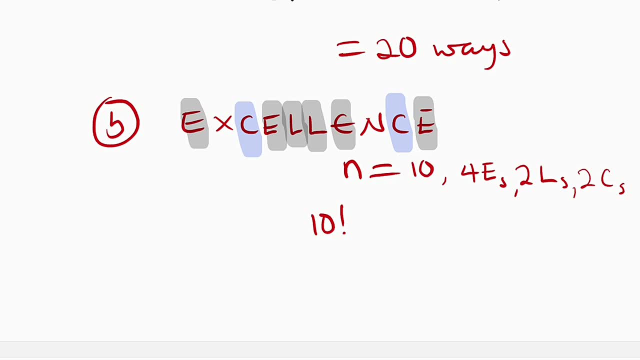 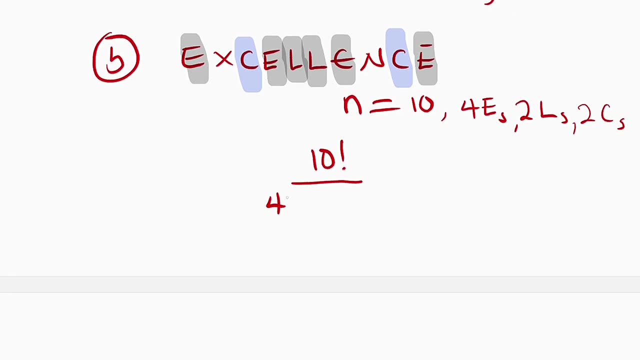 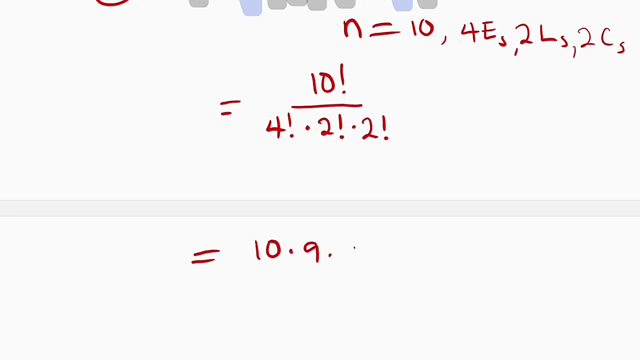 have to divide by the number of ways we can arrange four e's and two L and two C's. so divide by four factorial multiplied by two factorial multiplied by two factorial. now let us simplify this. if you simplify this, you have 10 multiplied by 9, multiplied by 8, multiplied by 7, 6, 5, 4, 3. 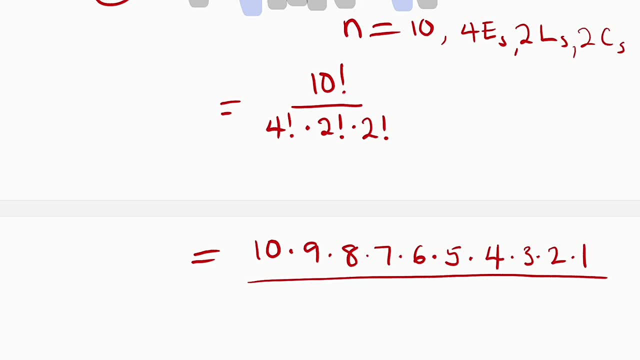 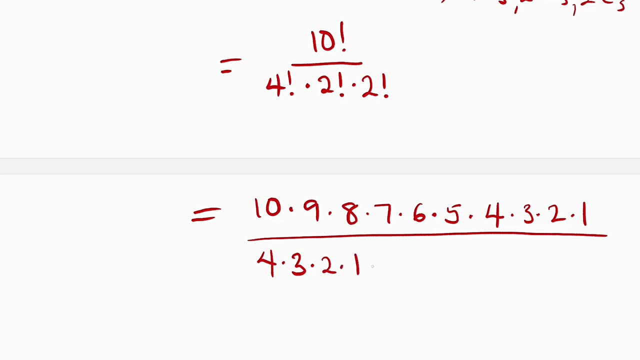 2, 2, 3, 2, 1 divided by 4, 4 factorial, we have 4 multiplied by 3, multiplied by 2, multiplied by 1, then multiplied by 2, factorial is 2 times 1. 2 factorial is also 2 times 1. so now let us perform. 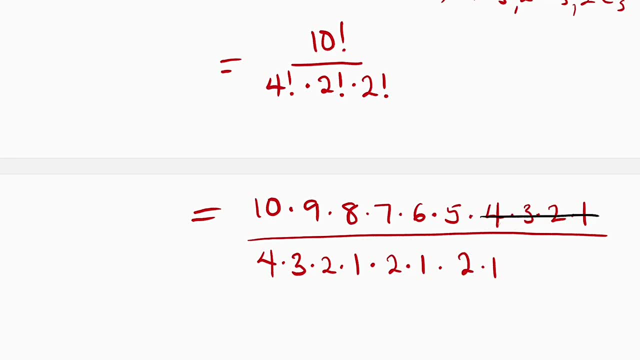 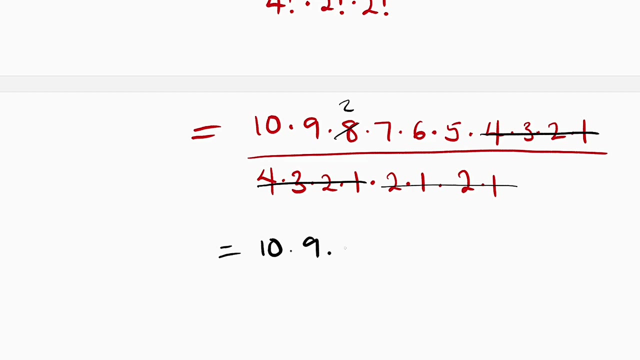 cancellation here. from 4 down to 1, we have 4 down to 1, we have 2 times 1 times. 2 times 1 is equal to 4 and the whole of this 4 can go into. each of these four evolves into 8, 2 times. so what we have is 10 multiplied by 9, multiplied by 2. 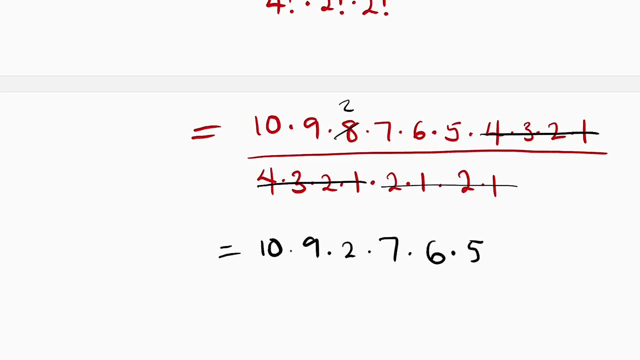 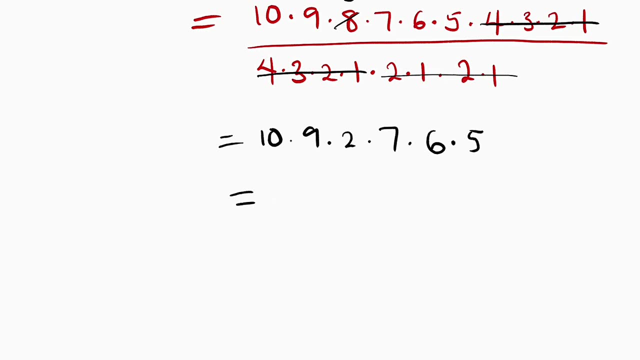 multiplied by 7, multiplied by 6, multiplied by 5.. Use your calculator and multiply all these numbers together to get the total number. If we can arrange the word excellence- and this is equal to 37,800 different ways of arranging the latest of the word excellence, and then the code mental unit is equal to the number of. 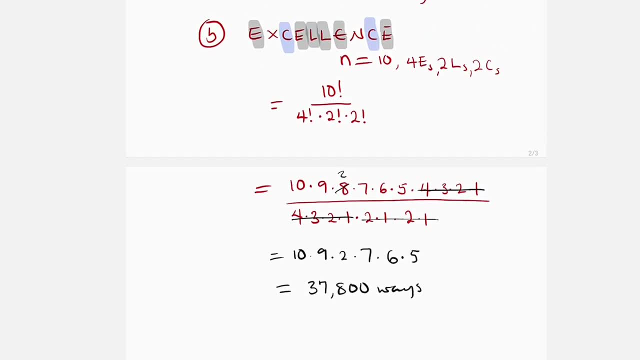 starts вариант of tooth weight lossèce of the word excellence, and the standard was F by zero. this is all I have for you today. Thank you for watching. Do share to your learning colleagues and don't forget to subscribe to my YouTube channel for more exciting videos. Bye-bye.